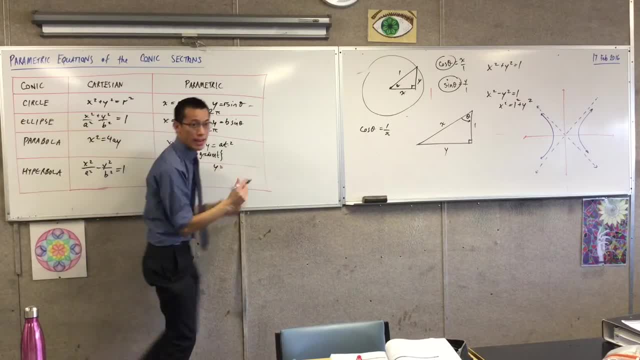 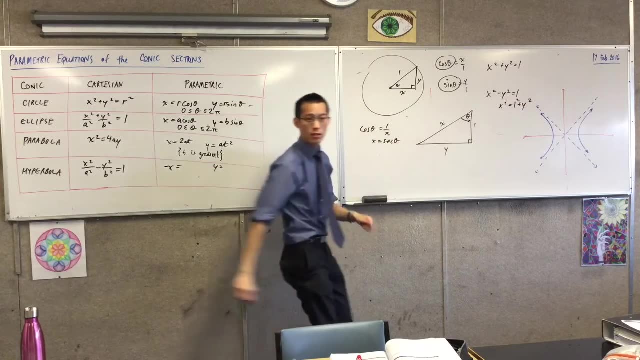 but I'm trying to head towards parametric equations. I'm trying to head to x and y equals. So I need to take reciprocals here. Do you see that? So really I would say x equals sec. theta Agreed, So that's good. 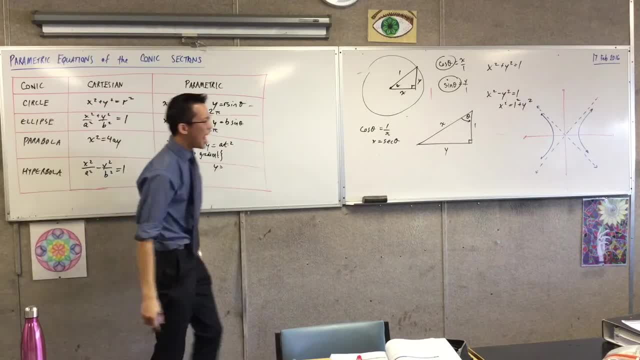 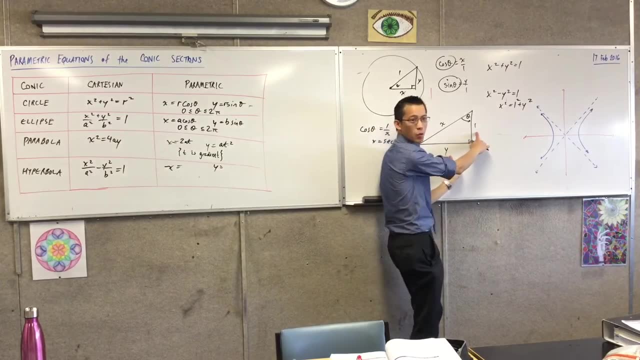 So now I've got a relationship. I can put it here: How about y? What would be a handy thing to get a relationship with y? I probably want to relate it to 1. I don't want to mix it in with the x. 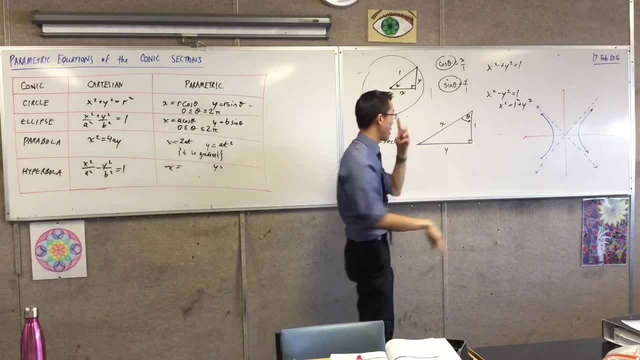 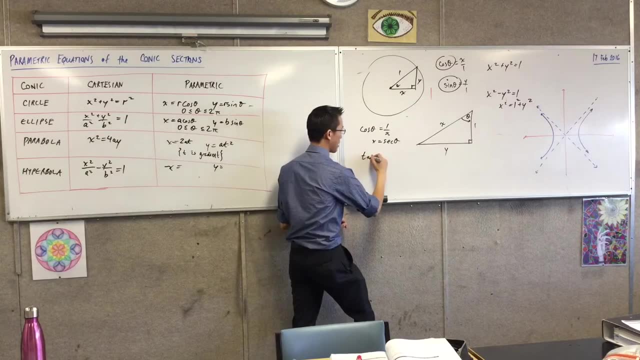 The whole point of parametric equations is to separate x and y out. So I want to relate these two and the ratio I would choose is opposite on adjacent, which is tan. So I would say tan theta equals opposite on adjacent Right. 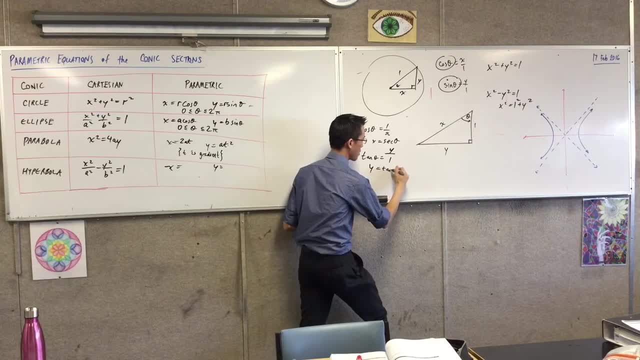 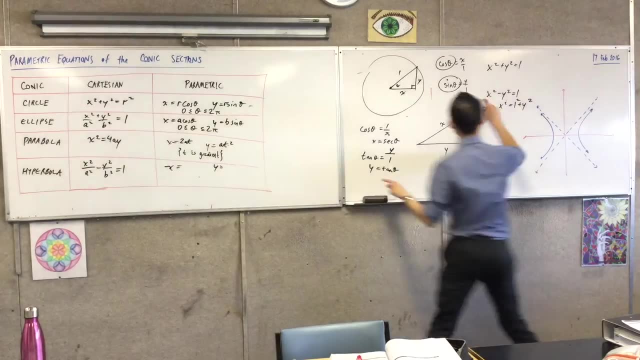 Does that make sense? So y is just tan theta. Does this make sense? Now you have a look at this. Is this going to check out sec theta and tan theta? Is it going to check out here? And the answer is absolutely. 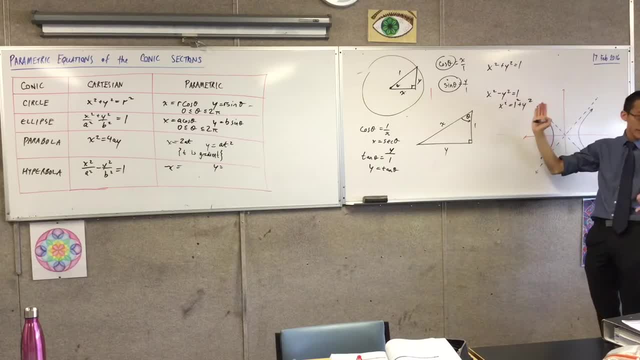 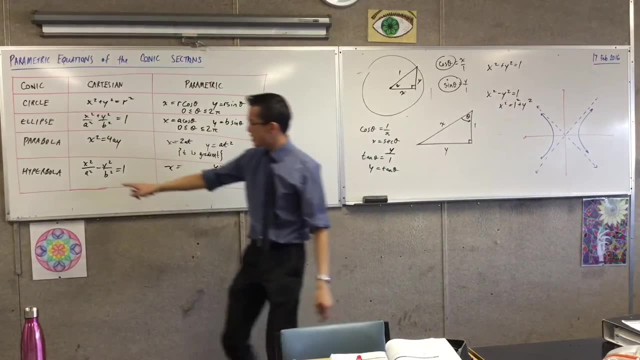 because sec squared minus tan squared is equal to 1, which is brilliant, just like we saw before with this one, the simpler version. All I need to do to get it over here is to say: well, I need to scale it by this amount for x. 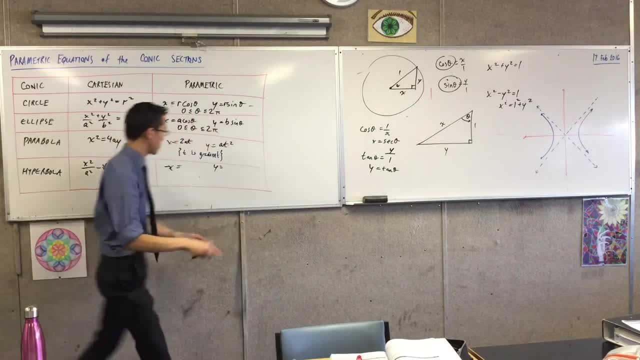 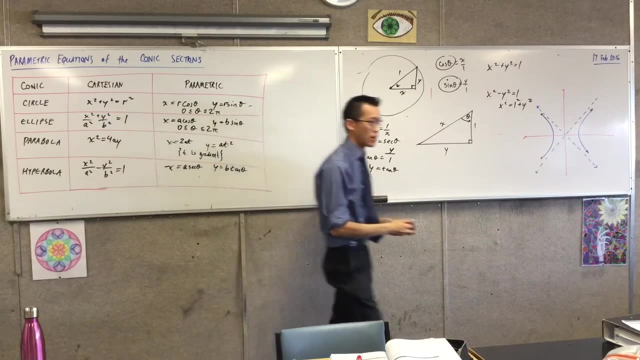 I need to scale it by that amount for y. Does that make sense? So I'm going to have a sec theta and b tan theta And I'm going to use tan theta as my parametric equations. Now one last little piece. 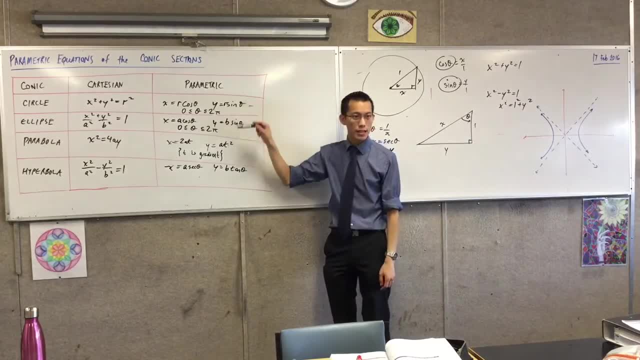 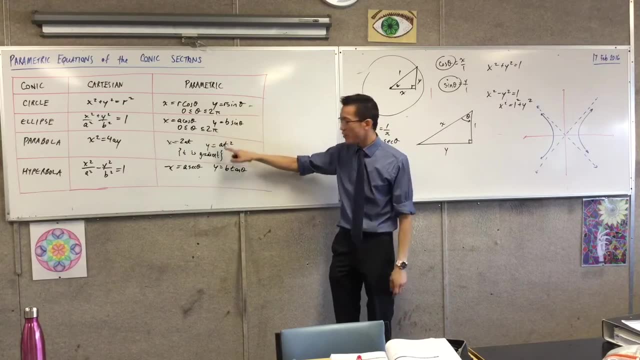 There's a bit of a problem when we look at the domain for theta, because remember we said theta can't just be anything you like. Now this in theory it could work, but really it's kind of a poor choice when you have a look at the function. 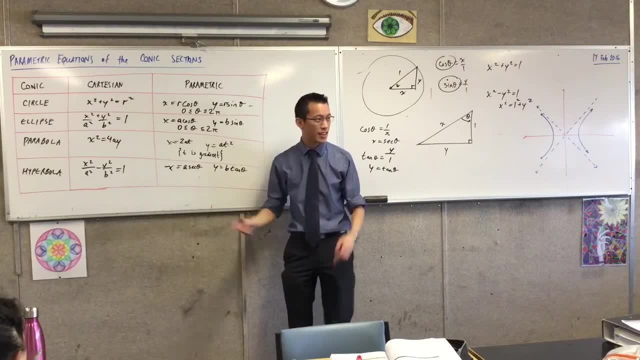 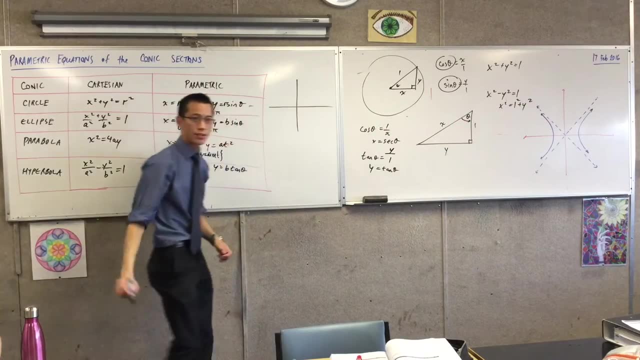 that you're dealing with, Because when I've got sec theta and tan theta, where do you want them to exist? Think about this: What do the graphs of sec theta and tan theta look like? What is this? Where's sec theta? 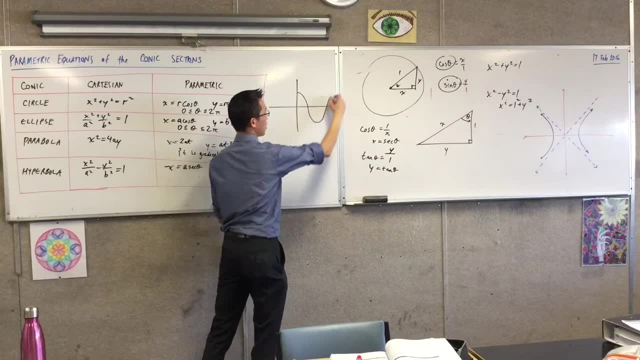 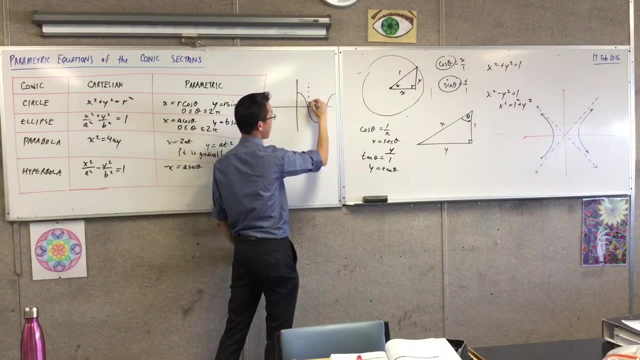 Like that bit. Yeah, this way, Here's cos right, So you can see. up until here it exists, right. So you're like, okay, at that point I'm going to get a vertical asymptote. So when I draw in sec, theta is going to look like this and like this: 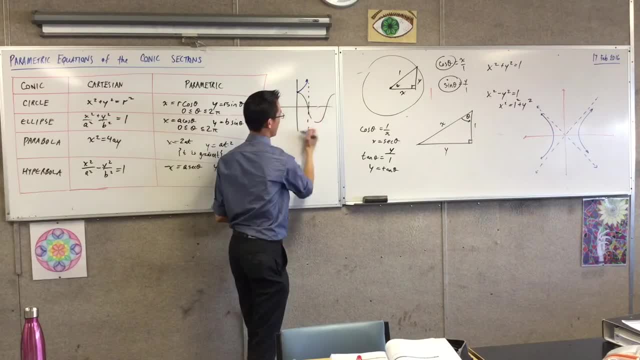 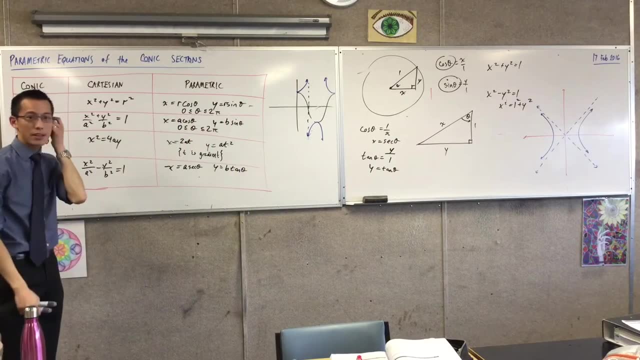 Do you agree? I could keep going, I suppose. So it starts from the bottom Down here, like that, Like so Is that okay? Now you have a look at this right Now. this is okay, but it's a little bit messy. 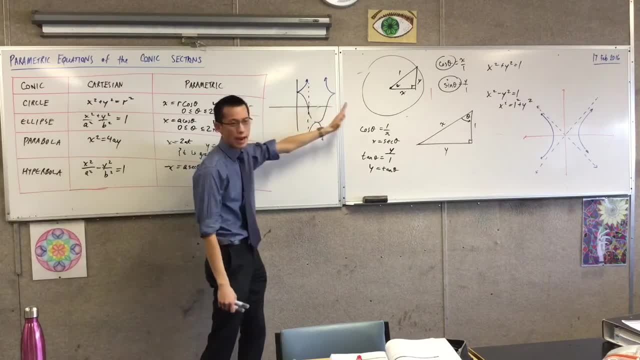 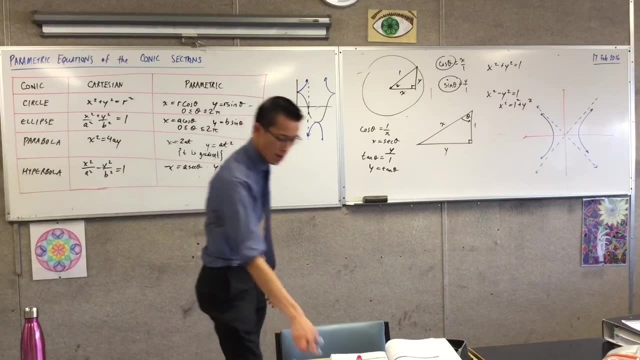 because now I've got like parts that overlap Like north of 2 pi. it's a bit gross. So therefore, again by convention and to try and deal with the different kind of symmetry that the hyperbola has, rather than going around in a circle. 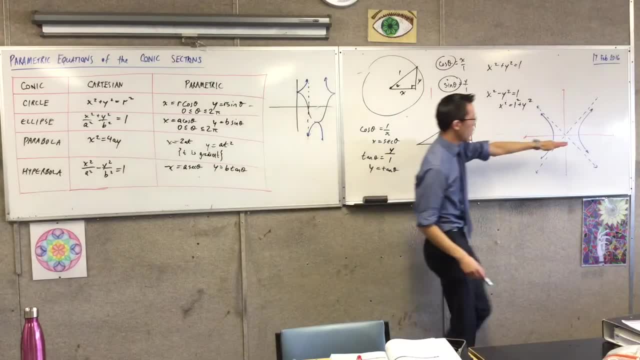 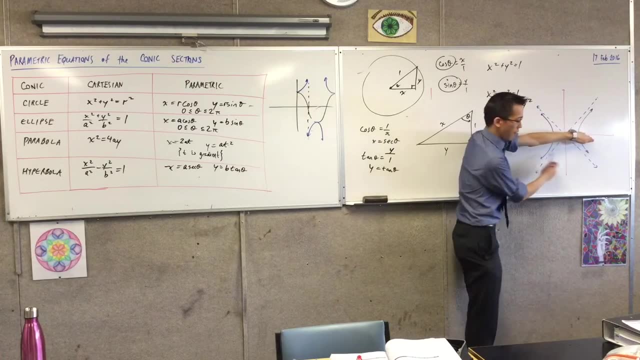 like it makes sense for a circle or an ellipse. instead we say: well, let's start from here, deal with the positive side up here, the first and second quadrants, and let's deal with the third and fourth quadrants separately. So we go from north to pi and we also go from north to negative pi. 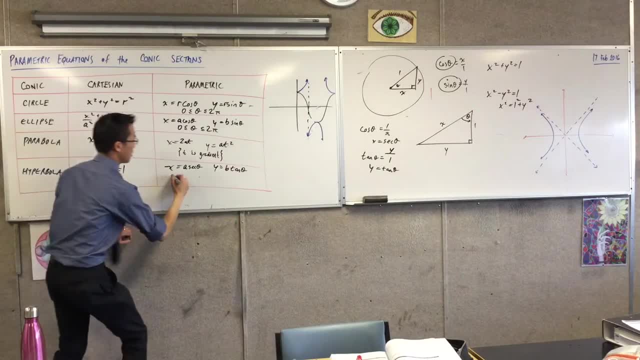 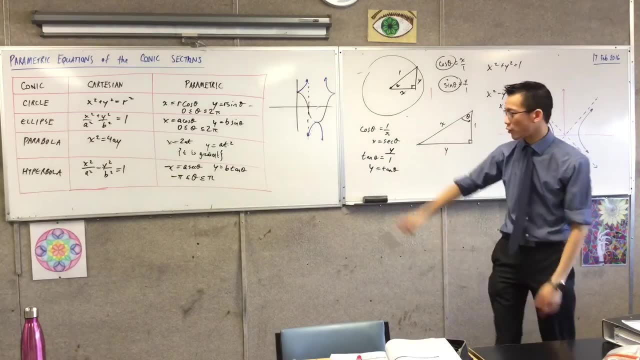 So I guess, doing that in order, we would say it has negative pi less than or equal to theta, which is less than or equal to pi. Now again, in theory they could have, and I've got some discontinuities in there. 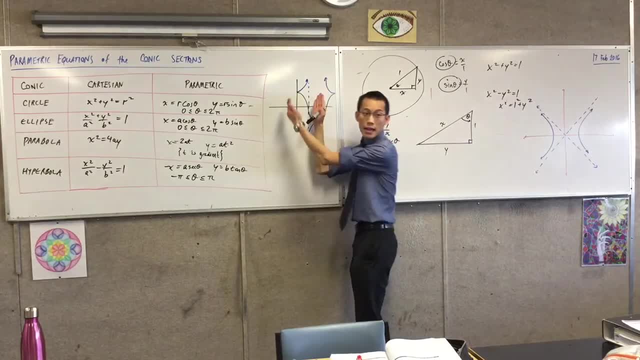 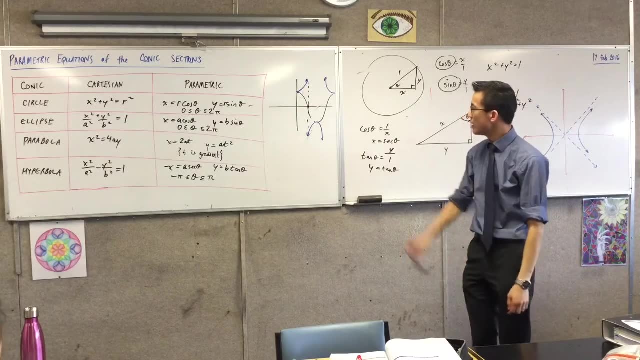 pi on 2 and negative pi on 2, like this guy and this guy. but you cannot avoid the discontinuities. There are always going to be discontinuities on a shape like the hyperbola. Now why do we use these? 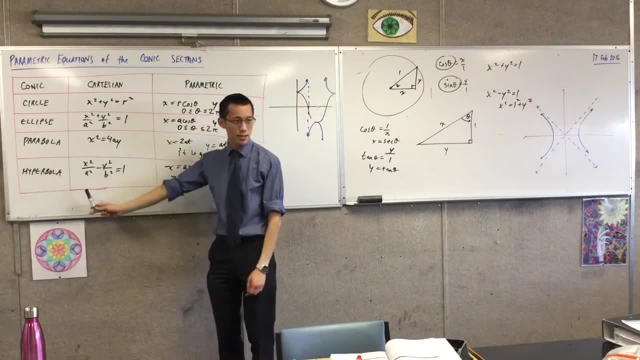 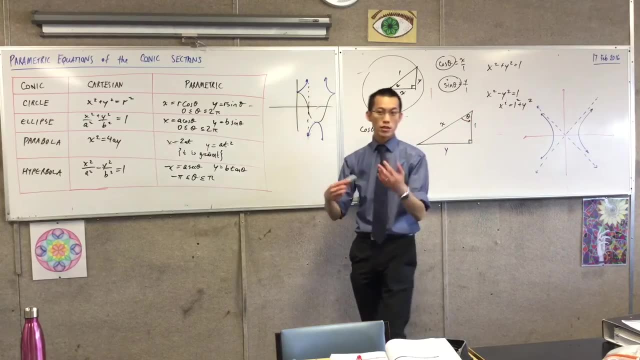 Why does this seem complicated as compared to this? And the idea is that, for instance, if you have a look at our shape here, there are going to be a whole bunch of points that behave in concert together. I'll give you a very simple example. 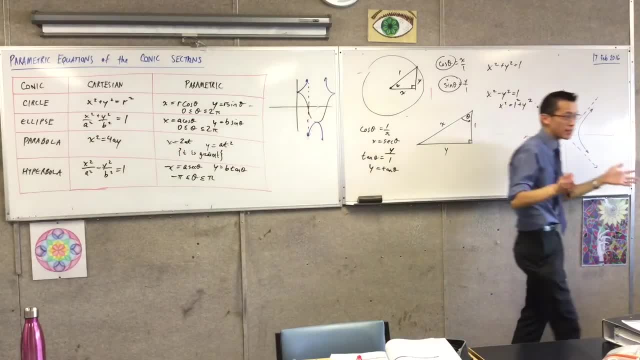 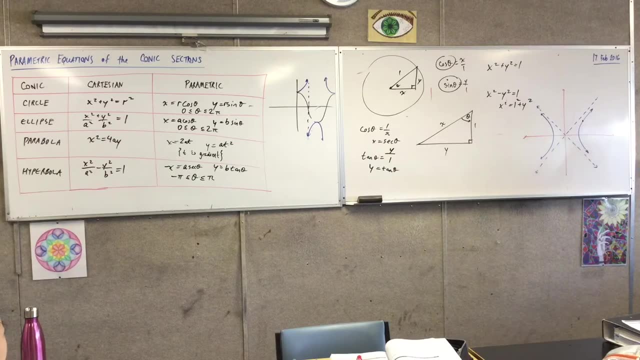 There's a whole bunch of pairs of points on the hyperbola where I can say, as an example, the tangents are going to be parallel. So, for instance- we've talked about this before. this is the reason why gradient is a poor choice of parameters. 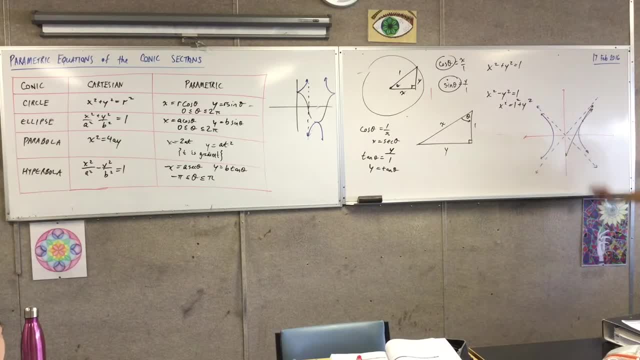 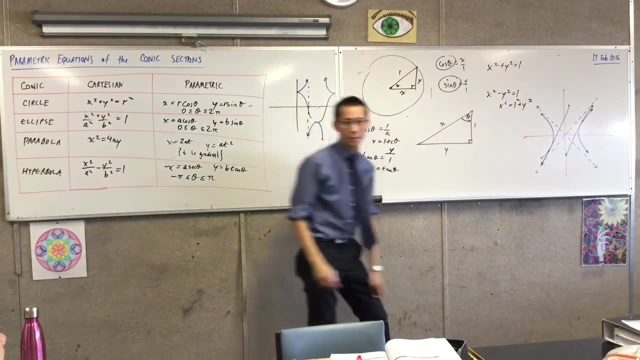 Right. So I'm going to draw a line there like so, That might be the tangent, And it's going to have a corresponding one somewhere over here, like so. So they look pretty parallel, don't they? Now, they're not the only ones. 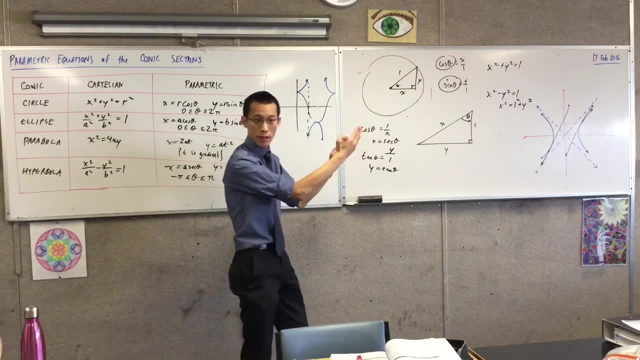 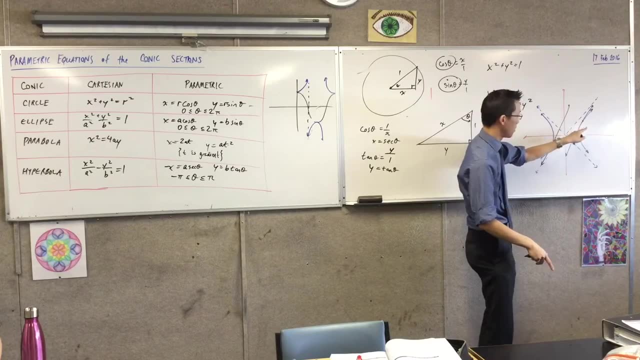 There's an infinite set of other points that will still do this parallel thing, and I can keep on moving. Now the key is, if I want to move around and understand how these two points relate to each other, an angle makes perfect sense to make a comparison between these two. 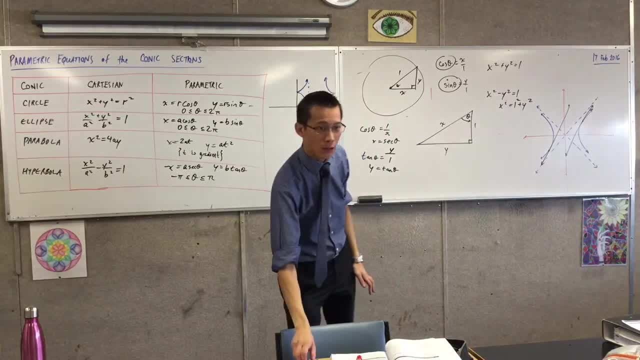 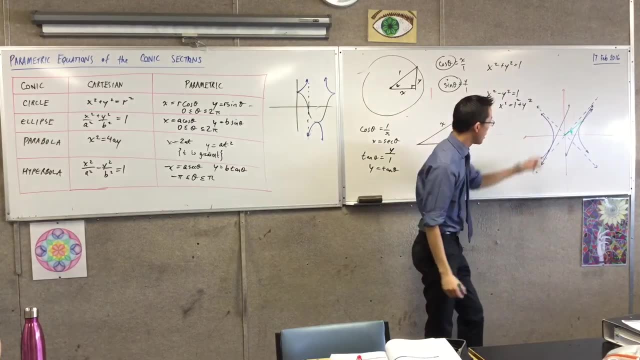 I mean in this example, can you kind of see what's the difference between the angles? Look, if I do that from the origin, if I go up to here, you have a look at that angle, And then if I go over here to the other point, 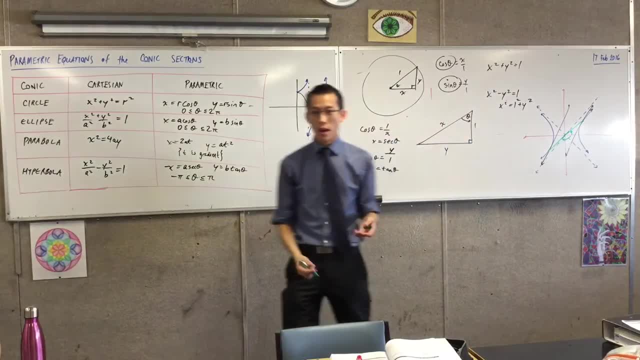 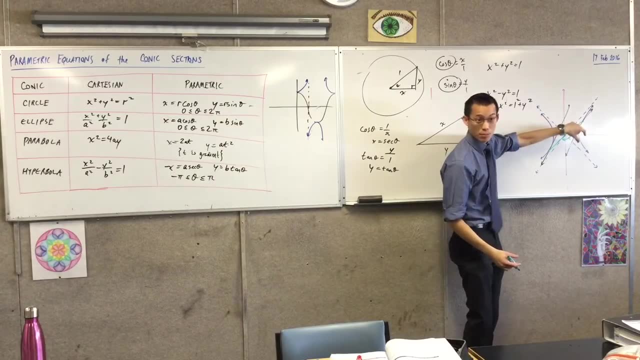 you have a look at that angle, What's the relationship? They are supplementary, aren't they? So just in one fell swoop we can see a clear algebraic relationship between those two. It's very obvious to see, provided you have a parameter to talk about it with. 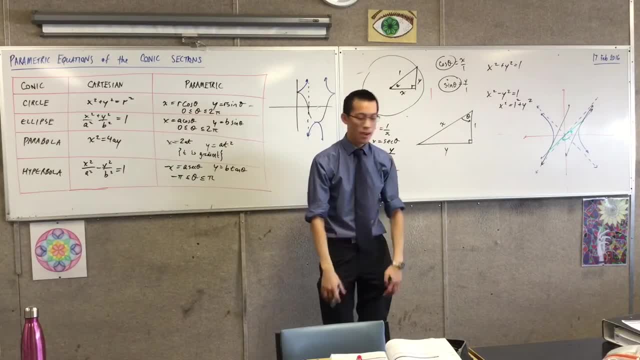 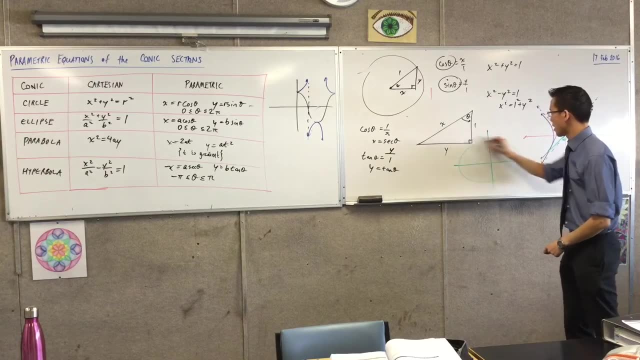 Now the downside is the algebra ends up being substantially worse. For example, I will come around and show you in a minute. Do you remember? there was this question right To prove that from one focus to another, that that distance there always is 2a. 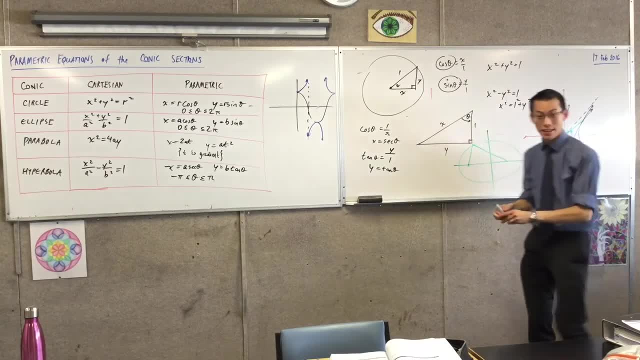 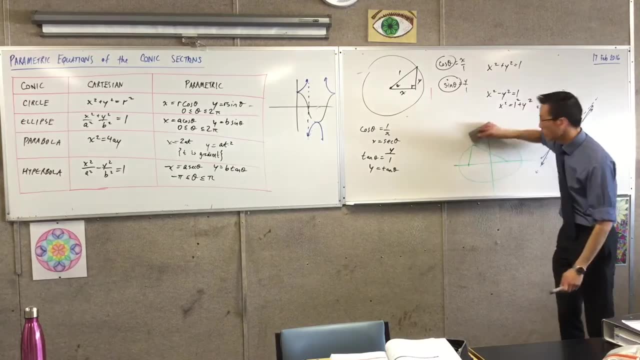 Do you remember that question? Now, there's a hard way to do it and there's an easy way. Algebraically, the hard way is with parameters. It's like ten lines of hard algebra. A much more beautiful way would be like this: 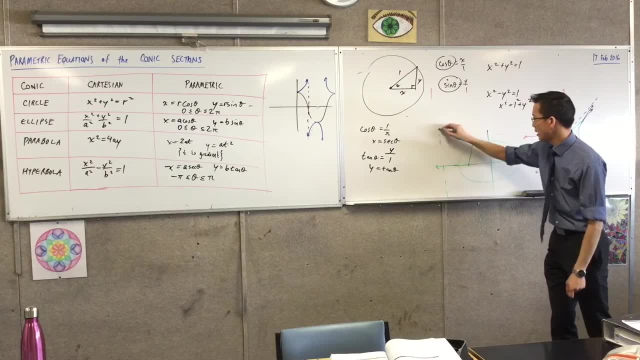 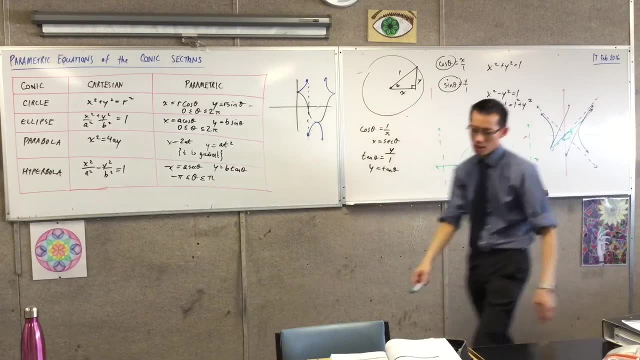 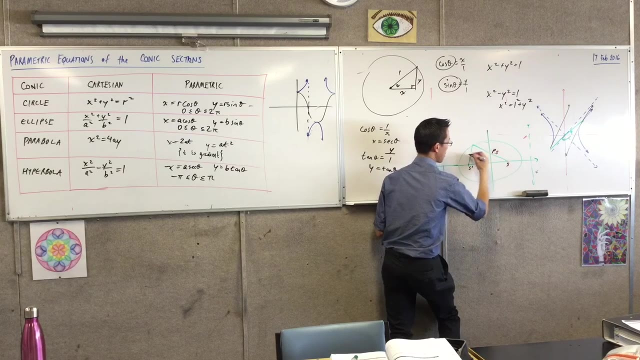 Watch. So you've got a directrix over here and you also have a directrix over here, Agreed. Now I've got here, say, for instance: I guess that would be s and s', so you've got ps and ps'. 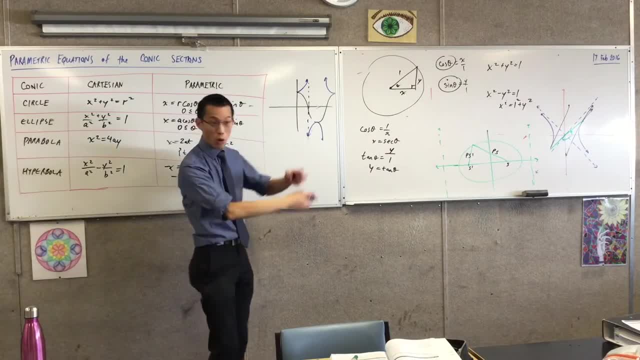 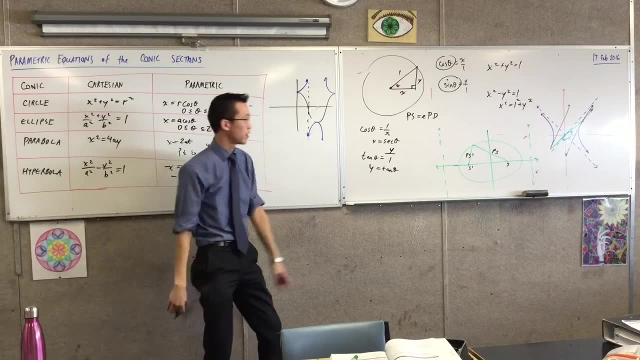 Do you agree with that? But by definition, because in all conic sections you have this relationship. That's the relationship that makes it work, and you put different values for e, you get different conics. Therefore, where are these guys on this diagram? 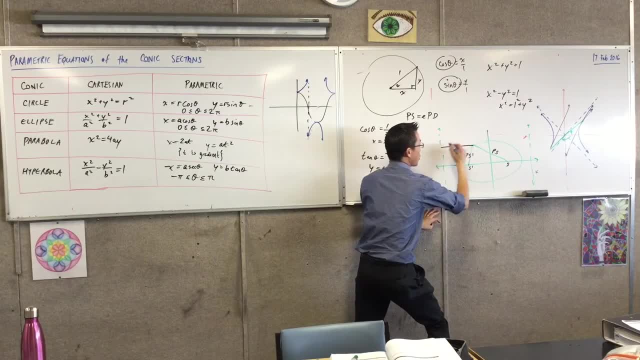 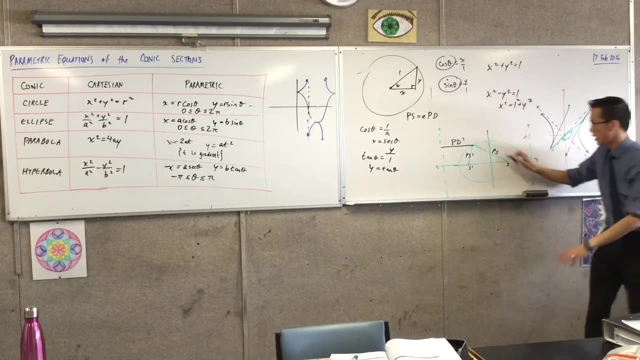 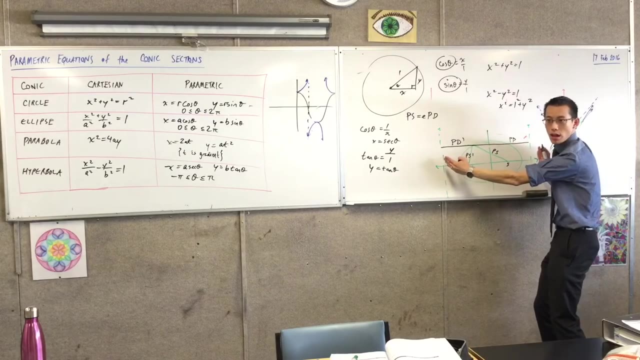 Well, this is ps'. pd' is over here, right? This is the corresponding directrix. And then pd, just regular pd, is going to be over here. Do you agree with that? But hold on a second. What are the equations of these two lines? 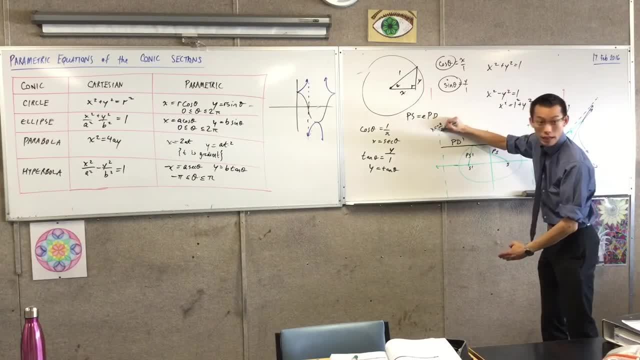 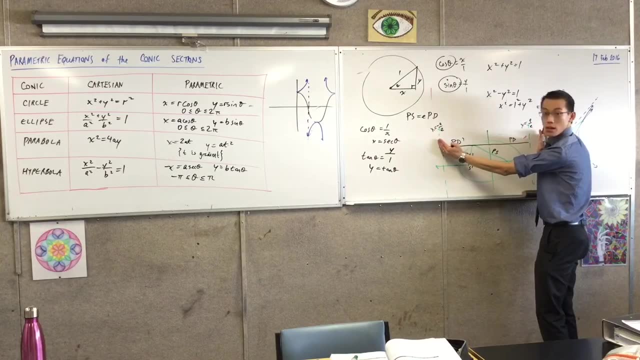 The directrices right, This is: x equals negative a on e and x equals a on e, right. So what is this total distance? 2a on e. So there's an a on e and there's another a on e. 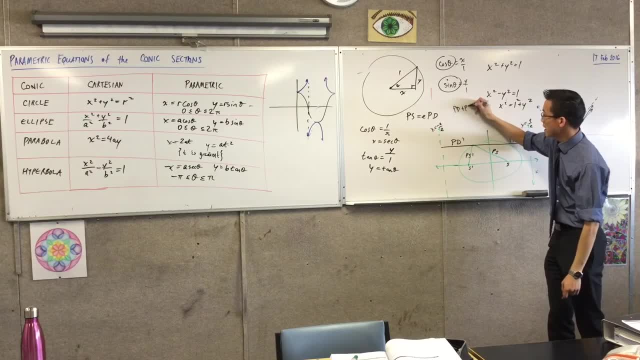 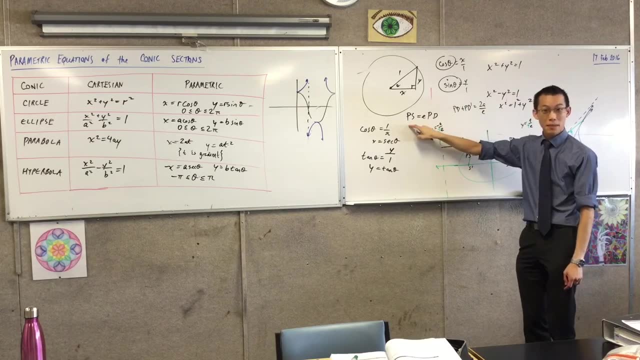 so therefore that total distance pd plus pd' equals 2a on e. I don't want pd on pd', I want ps plus ps' right? The difference between those two is a factor of e. So if you put an e outside there,